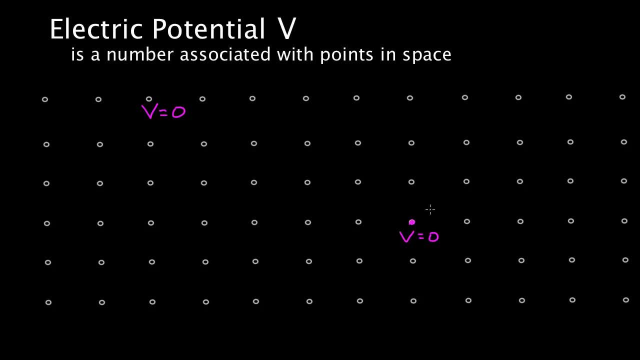 The number associated with every point in space would be zero. that'd be boring and useless. How do we make it so that the V value, the electric potential value, is not zero? We'll just stick a charge in here. So let's take a big old positive Q. 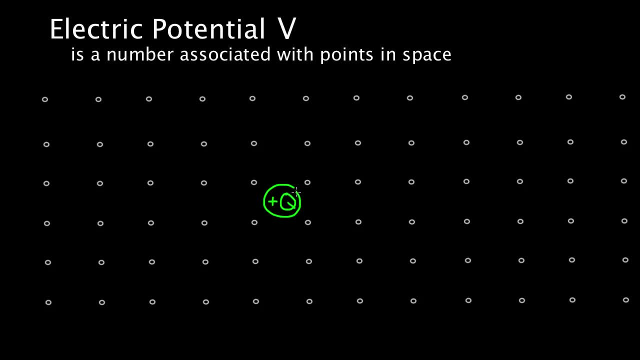 at some point in space over here, Pick a big old charge and we'll stick it right there. Now points in space around this charge will have a V value that's non-zero, And they'll be big if you're near this Q. 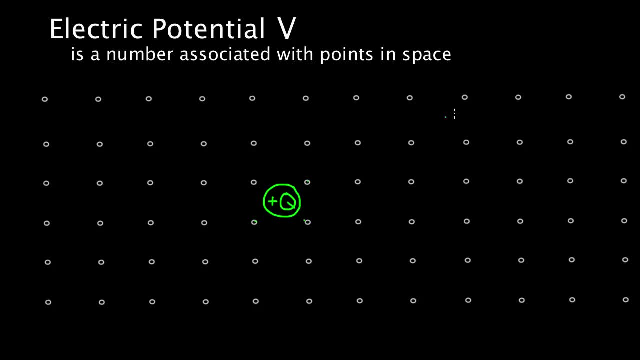 So the V values around here are gonna be really big, And then the V values way out here will be smaller. The farther away you go, the smaller it gets. And why do we care? Who cares? The reason we care is this: 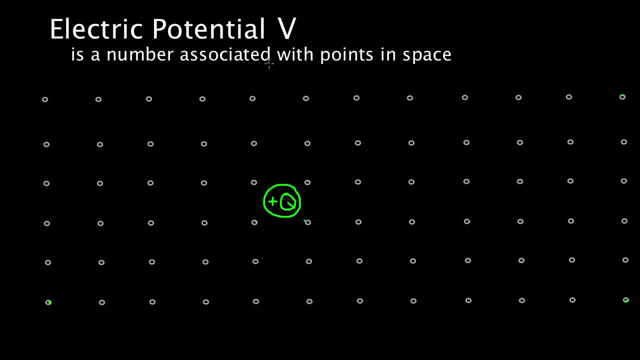 The units of electric potential are joules per coulomb, So electric potential has units of joules per coulomb. That gives you a hint of why you should care. We care about joules. Joules are energy, So if something can have energy, that's useful. 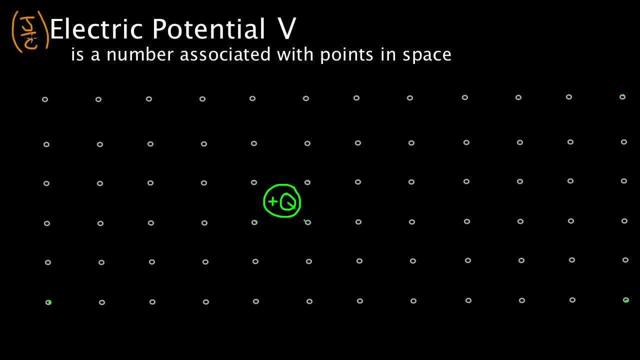 You can get work out of that or it can turn into kinetic energy And joules per coulomb. that lets you know. all right. well, if this point over here happened to have, say, 100 joules per coulomb, 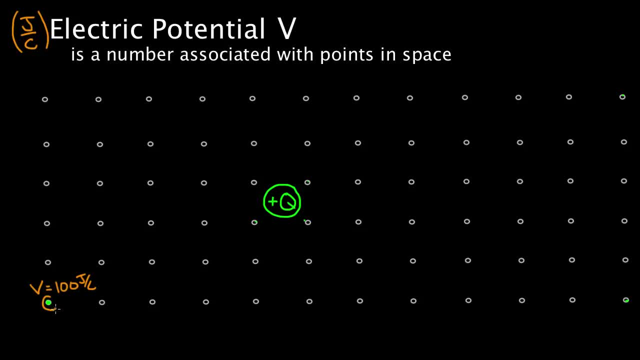 let's say the V value at this point in space happened to be 100 joules per coulomb. what that means is remember there's nothing there. But if there was something there, if we happened to take, say we had a positive two coulomb. 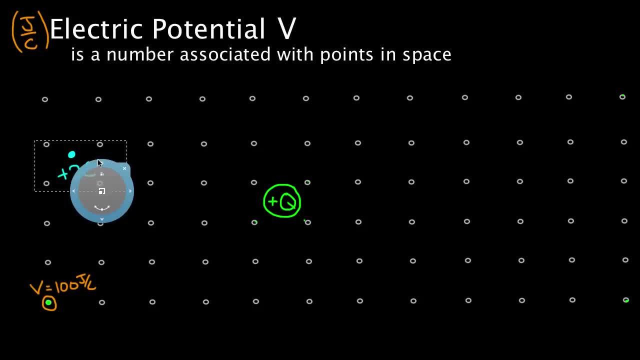 charge and we took that charge and we put it there at that empty point in space. before we put it there, the V value was 100.. When we stick it here, who cares? Why do we care about this 100 value? 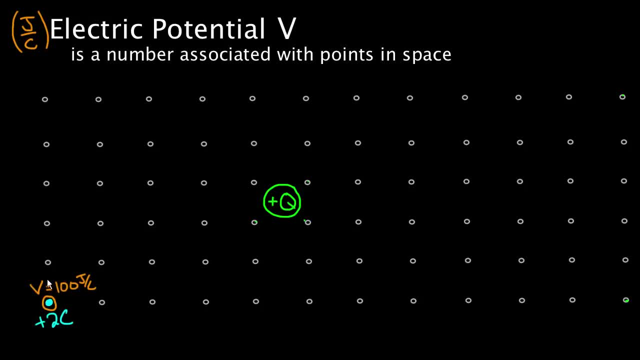 Because, look it, it's 100 joules per coulomb. That's what V the electric potential is telling us. So if it's 100 joules per coulomb, that's 100 joules per coulomb. 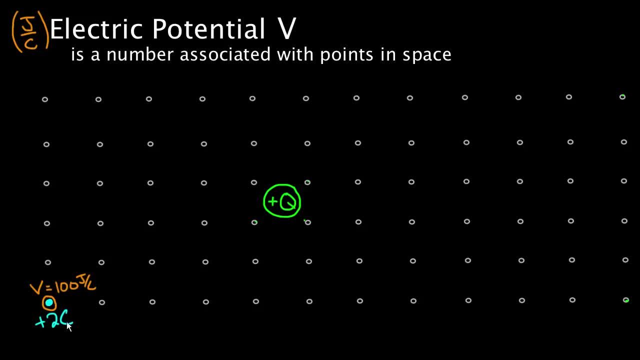 So if it's 100 joules per coulomb and I stick two coulombs there, how many joules of energy do you think it's gonna have? It'll have 200, and that's the key. That's why we care about electric potential. 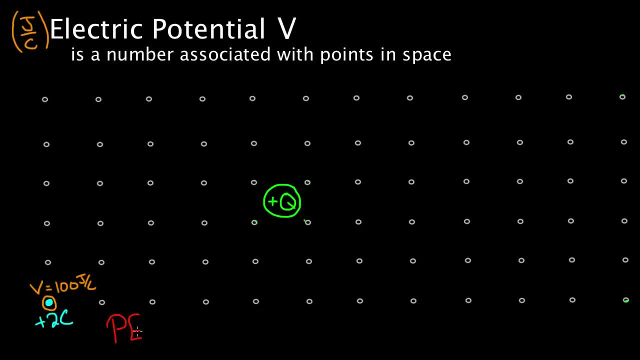 because it lets us find electric potential energy Either P-E. sometimes people write electric potential energy as U, So the formula is just: Q, you take the Q that you stick at that point in space. in this case it was two coulombs. 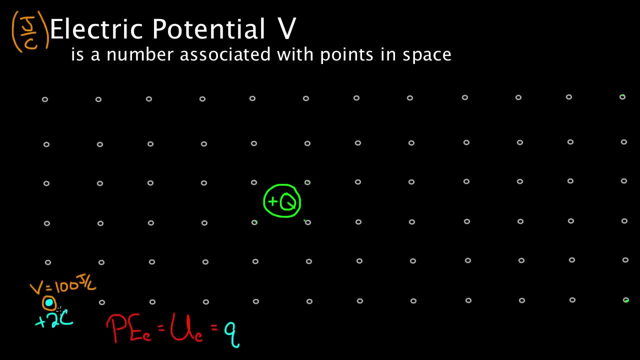 take whatever Q there is, multiply it by the value of the electric potential and that tells you how many joules there will be for the charges in that region. So this electric potential energy is between these two charges. here the charge that created the V 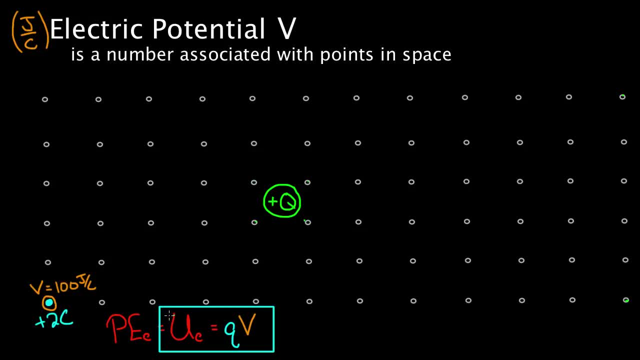 and the charge that you stick at that point, and the V is a quick way to figure out how much potential energy- electric potential energy- there would be. So, in other words, in this case, since I had two coulombs there, I'd take my two coulombs and I'd multiply by 100,. 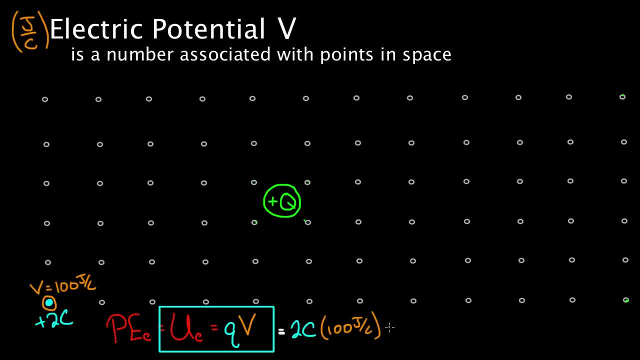 the joules per coulomb, because that's the V value and I'd get that there are 200 joules of potential energy now stored between these charges. So that's why we care about electric potential V. It's a way to figure out the electric potential energy. 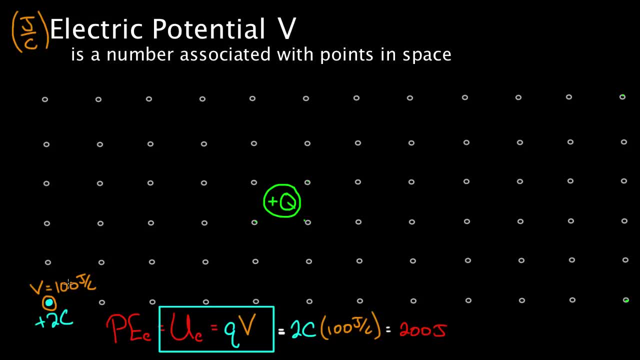 for a charge that's placed at that point in space that has that V value. But how do you get this V value? If I hadn't given you the 100 joules per coulomb, we wouldn't have been able to figure this out. 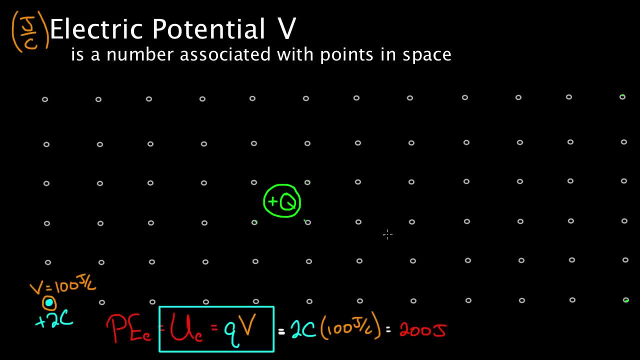 We need a way to figure out the V value at points in space based on the charges creating them, because charges create the V value. There's a formula for it and the formula says that the V, the electric potential created by point charge, is equal to K. 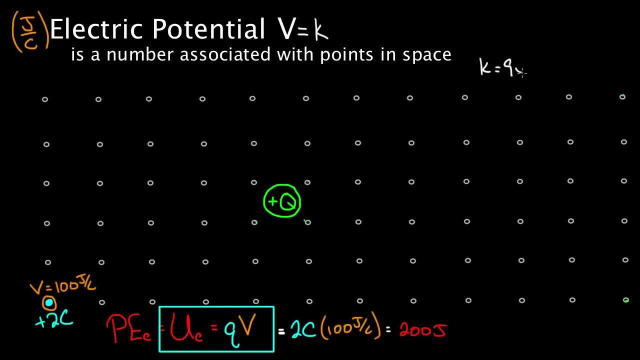 K is the electric constant nine times 10 to the ninth, and it has units of Newton meters squared per coulomb squared. so that's always K. You take that K and you multiply by the charge. that's creating the V value. so in this case it's this Q. 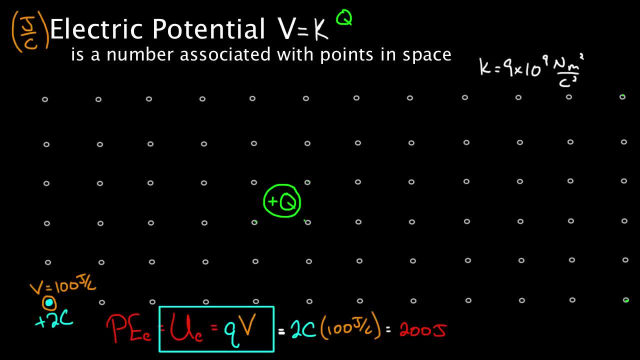 This positive Q here, whatever Q, it is creating the V value that you want to find, and that's key. If you plug in five coulombs here, you're finding the V created by that five coulombs. If you plug in negative, three coulombs. 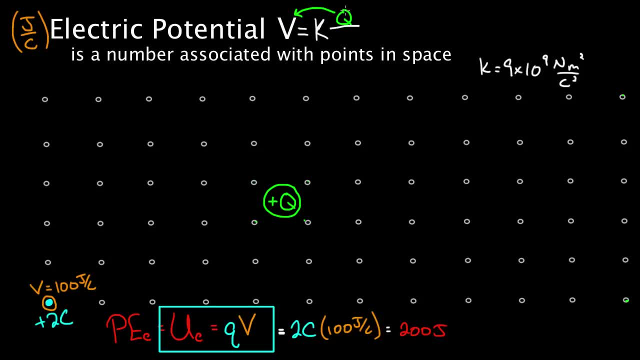 you're finding the V created by the negative three coulombs. Sometimes there's problems with multiple charges in it, like this one. and this Q has got to be the charge creating this V, Not the charge you placed at that point in space. 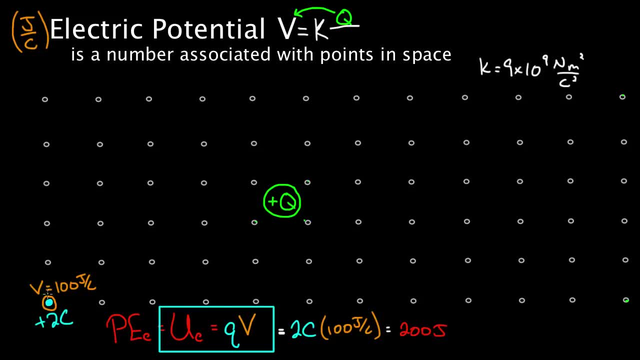 I don't put the two coulombs up here. I put the charge creating the V value that I want to find And then you divide by the distance. So I divide by the distance between this charge and the point in space that I want to figure out. 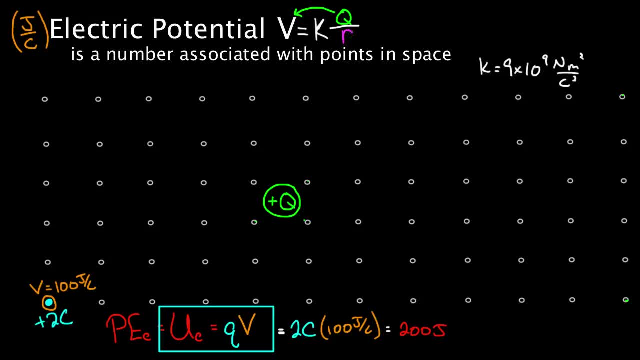 the V value at. Some people call this the radius. I don't like calling it. the radius Makes it sound like there has to be a circle. There doesn't really have to be a circle. This R would be the distance from this point. 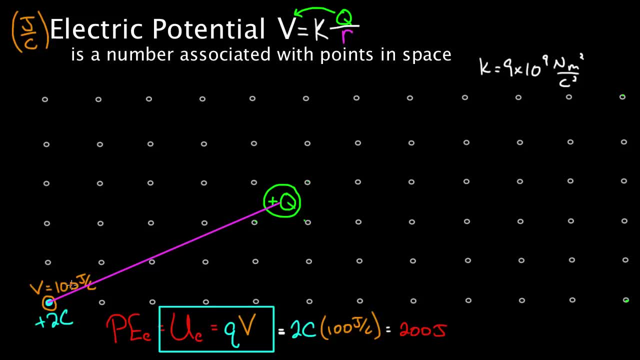 the charge creating this V value to the point in space where I want to determine the V value, That's R. So this is R. So how would we determine this? Well, let me just give you some numbers. Let's say the charge we stuck here was one nanocoulomb. 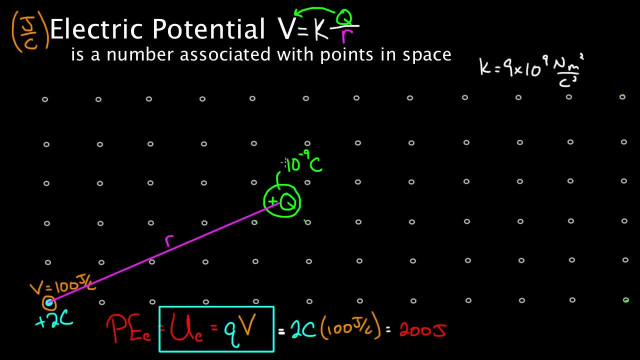 Nano is 10 to the negative ninth. So let's say that was one nanocoulomb And let's say the distance from this charge to this point in space was, let's say it was nine centimeters. And I want to know what's the V value? 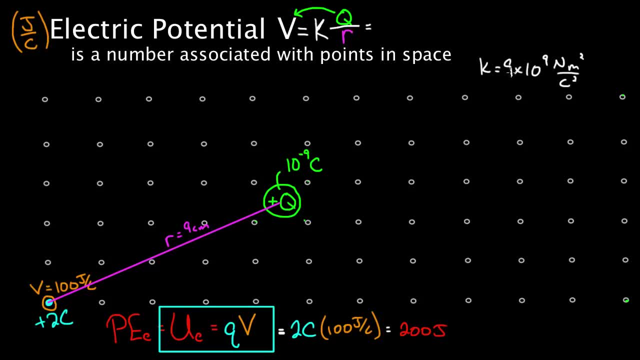 Well, I can solve for it now. We've got our formula. The V would equal all right. my K is nine, always times 10 to the ninth, And it's Newton's meters squared per coulomb squared. And then I multiply by my charge. 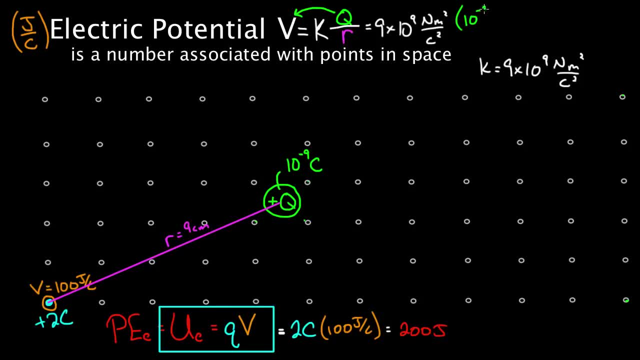 And I told you that the charge here was 10 to the negative ninth coulombs. This is a nine, And my distance I divide by the R value And the R value is nine centimeters. But be careful, everything's got to be in terms of meters. 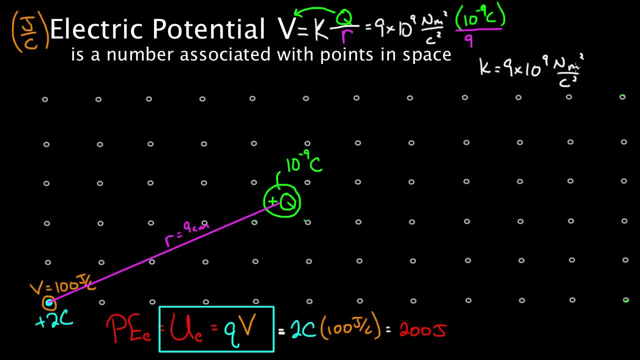 kilograms and seconds when you're doing physics with constants. Look at this: this is in terms of meters, So I've got to use meters here. So nine centimeters is .09 meters, And if I multiply all this out, what you'll get? 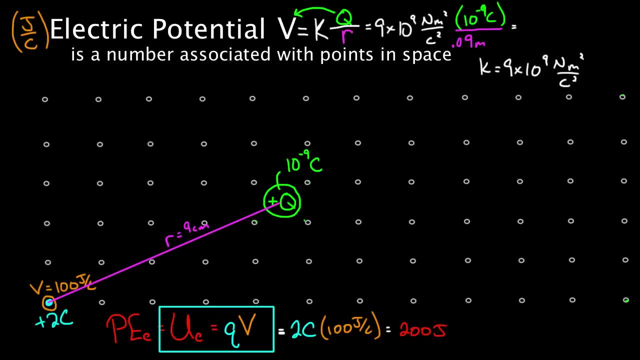 this 10 to the negative ninth cancels this 10 to the ninth By powers of 10, these just go away And then I have nine divided by .09.. That's going to equal 100.. So I chose this so that we got the same answer down there. 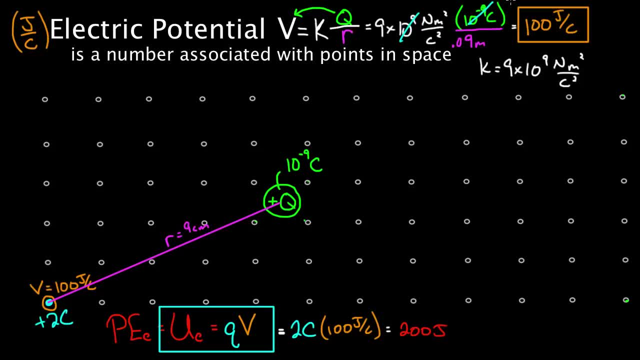 Get 100 joules per coulomb. You might be like: where'd the joules come from And how's this joules per coulomb? Well, let's look at it. If we took, look at one of these meters. 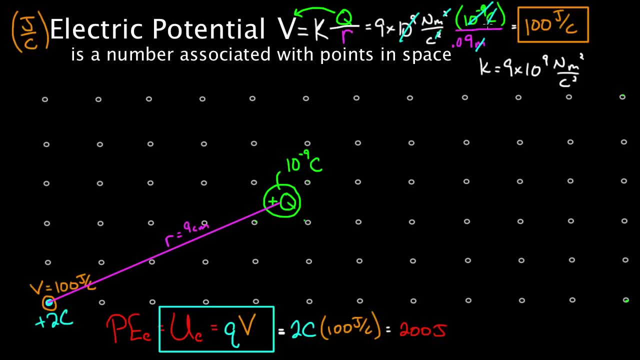 cancels one of these meters And one of these coulombs cancels one of those coulombs. What are we left with? We're left with Newton times meter over coulomb. But Newton times meter, that's force times distance. 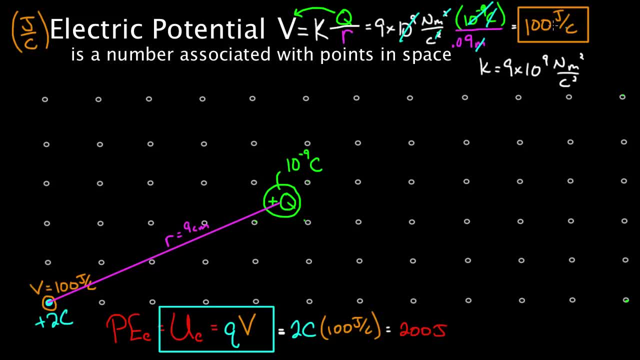 That's joules. That's where we get joules per coulomb, So this really does give us the number of joules. there will be at a point in space per coulomb of charge that you put there And it works for any point. 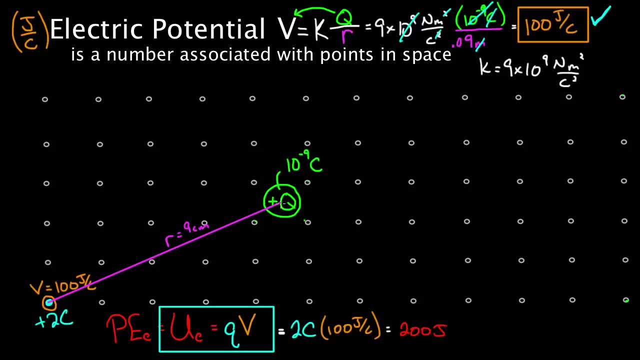 You pick any point. If I picked a point twice as close, that's half as far away. say some point over here. Let's say this r value here was only 4.5 centimeters. Well, I'm dividing this by r. 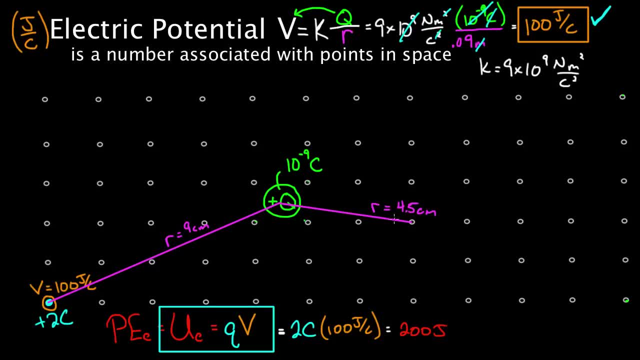 So if the r is half as big, this point is half as big. This point over here would have a v value of 200 joules per coulomb, And the closer I get if I went, even closer, if I went to a point that was 3 centimeters away. 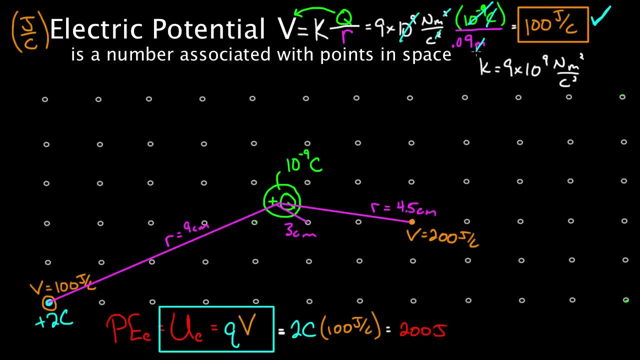 well, this is a third as much as this other distance. So if I'm only dividing by a third as much distance, I should get three times the result. This r is not squared, It's just r, So this point would have a v value of 300.. 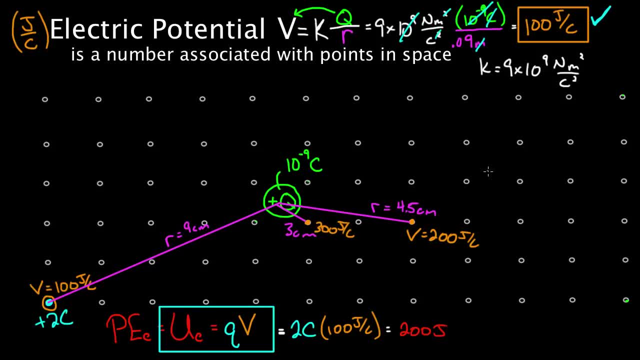 This would be 300 joules per coulomb. This tells me, if I wanted to get a charge to have a whole bunch of potential energy, I should put that thing nearby, I should stick it over here. This would give me a lot of potential energy. not quite. 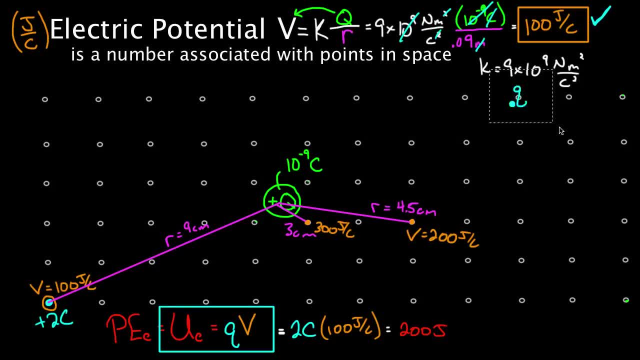 as much, even less. The farther I put my charge, the less potential energy it would have. There will be no potential energy until there is a charge. There will just be electric potential. But once you place another charge in that region to go with the first one, then you'll.